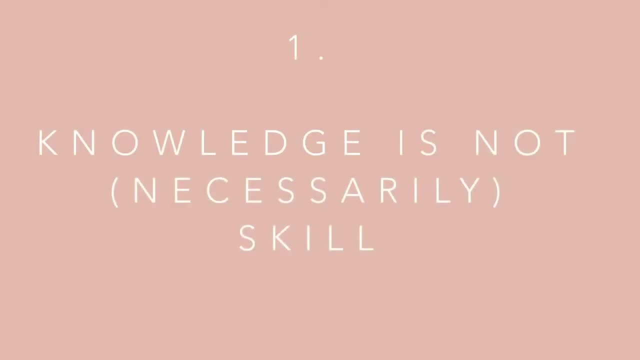 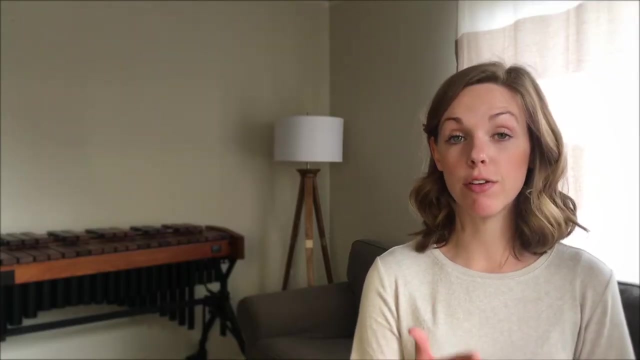 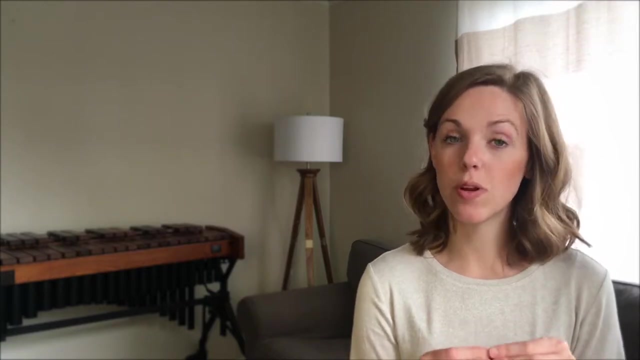 trial and error. So let's jump right in. So imagine giving your third graders a multiple choice quiz, maybe as an exit ticket, maybe as a paper and pencil assignment, And on that quiz, one of your questions is: which of the following rhythms is a sixteenth note? And then you list out. 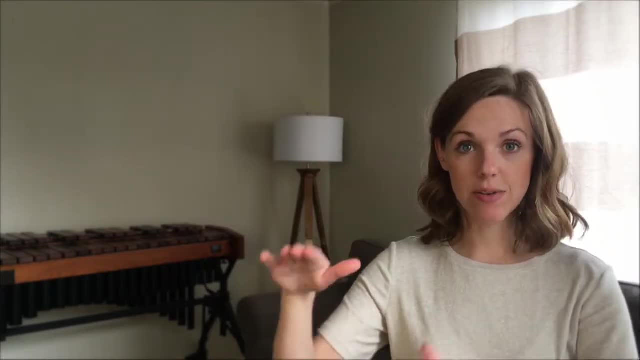 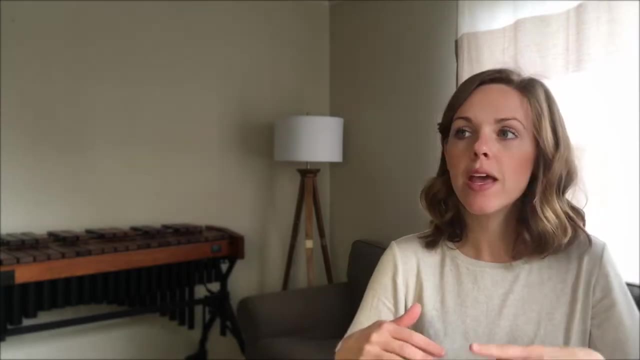 a quarter note, a half note, a sixteenth note and an eighth note, And students need to circle A, B, C or D. Which of the following is a sixteenth note? Now, a question like this can give you some. 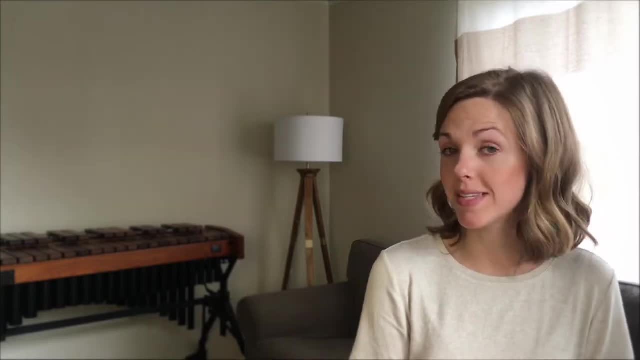 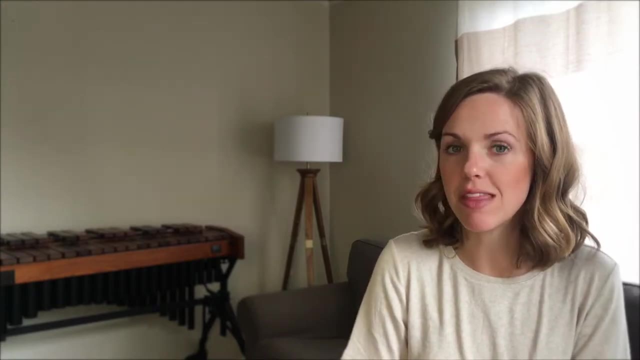 really valuable insight into what your students know about sixteenth notes. It tells you if they can recognize the shape of a sixteenth note. It tells you if they know the name of a sixteenth note, And both of those are really, really important things for us to know if our students 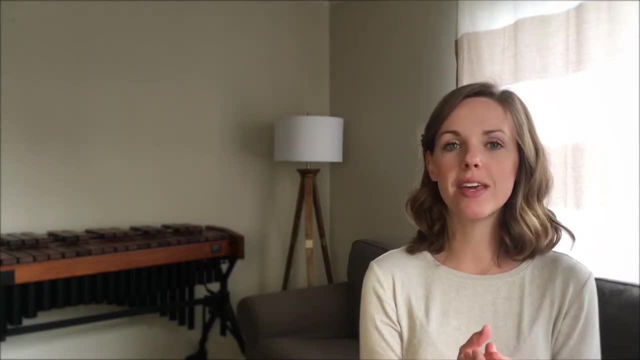 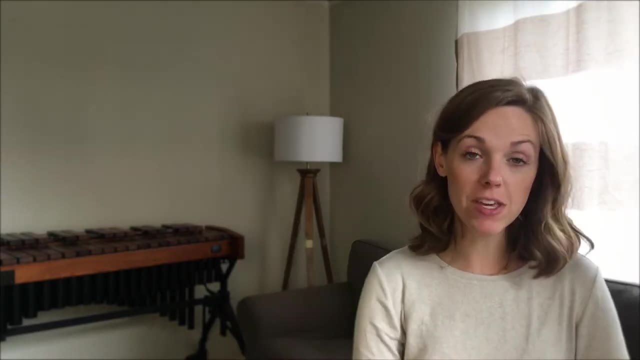 can or cannot do. But keep in mind that just because a student can recognize the shape of a sixteenth note does not mean necessarily that that student knows the shape of a sixteenth note. A student knows how a sixteenth note feels or what it sounds like or how they can use it in. 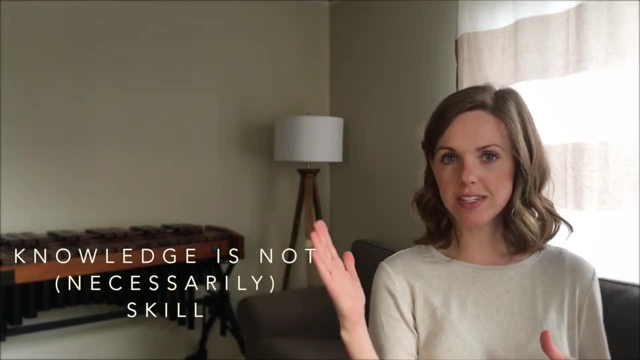 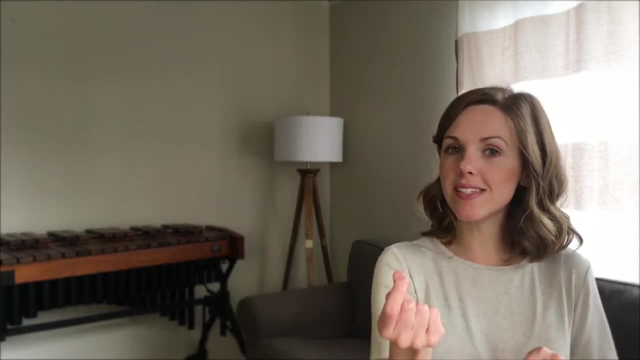 a composition. What I'm saying here is that knowledge does not necessarily mean skill, And assessing knowledge is a great thing to do, but you have to realize that when you assess knowledge, you are just assessing knowledge. You are not assessing what the student can do with. 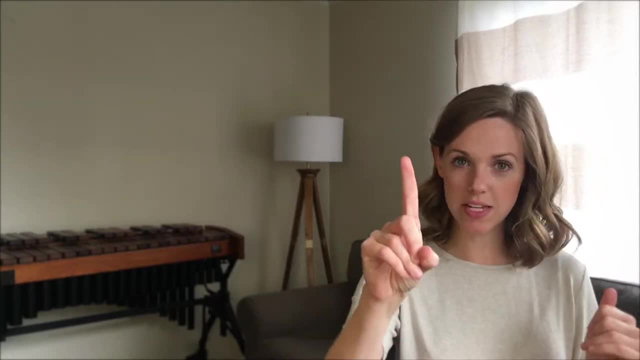 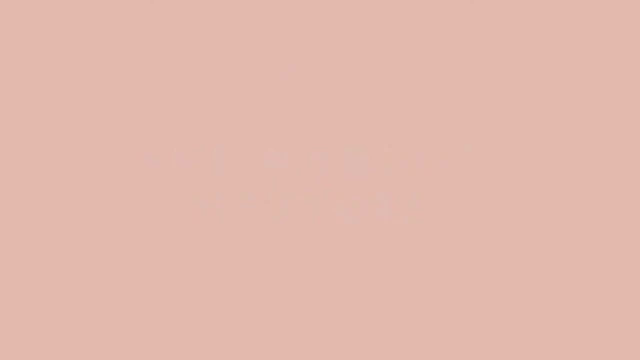 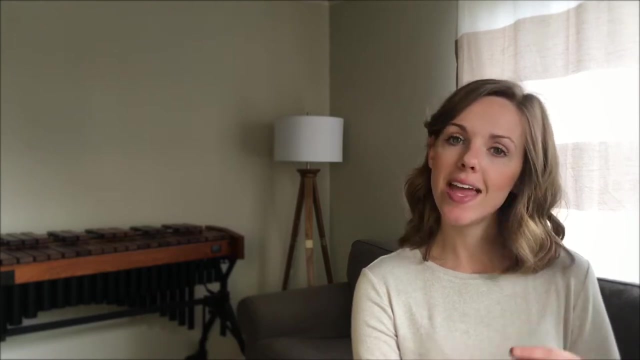 that knowledge Number one. we cannot confuse knowledge with skill. Number two: the medium matters. I once gave a really short multiple choice activity to a group of kindergartners and we were working on musical opposites, So high and low, fast and slow, long short, things like that. And in this activity 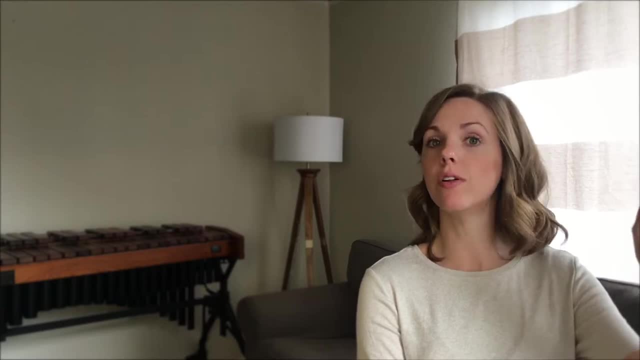 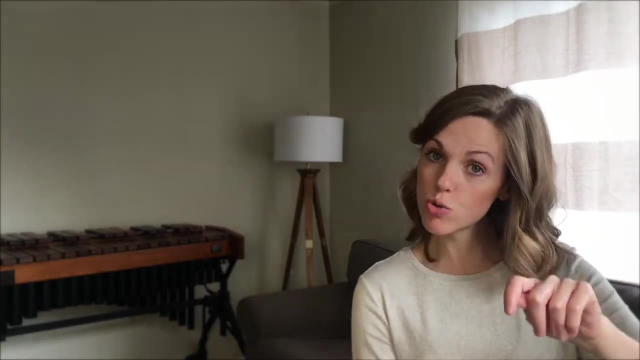 I was going to play a piece of music and students would circle if they heard high or low, And then they'd move on to number two. We would play a different piece of music. They would circle if they heard long or short, And it went on like that through about seven questions. What I didn't 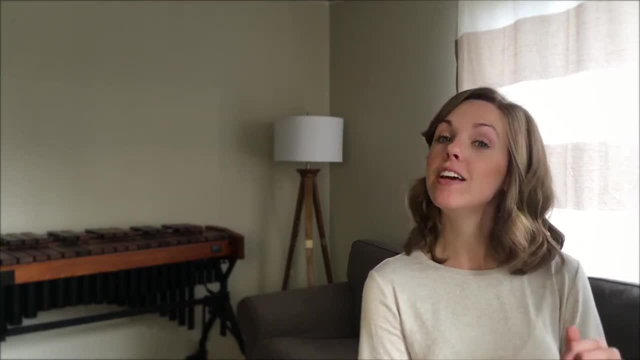 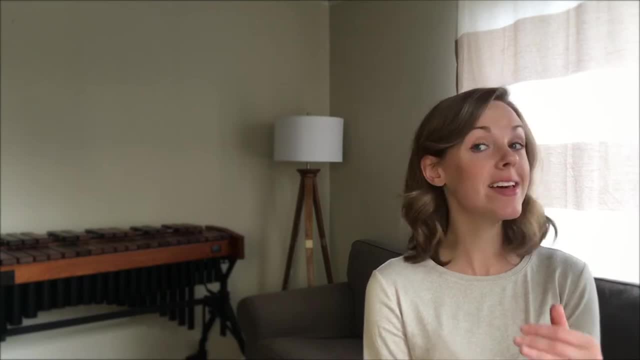 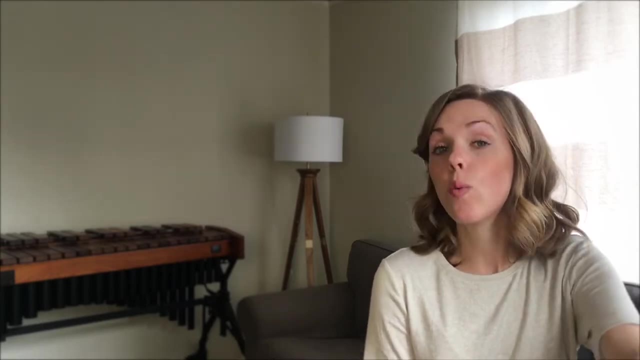 was asking them to show their musical knowledge in a way that didn't make sense to them. The worksheet I had created was way too complicated for them to actually be able to showcase what they could do with musical opposites. What I took up at the end of the activity was a mismatch of 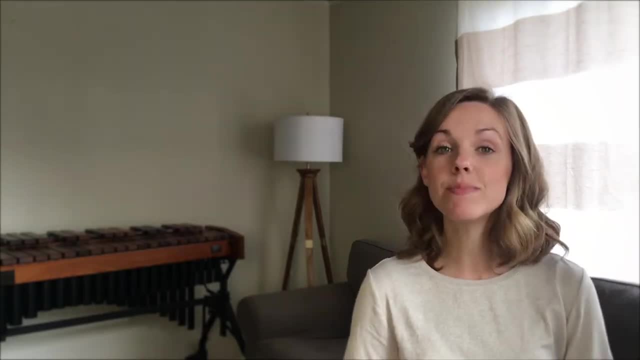 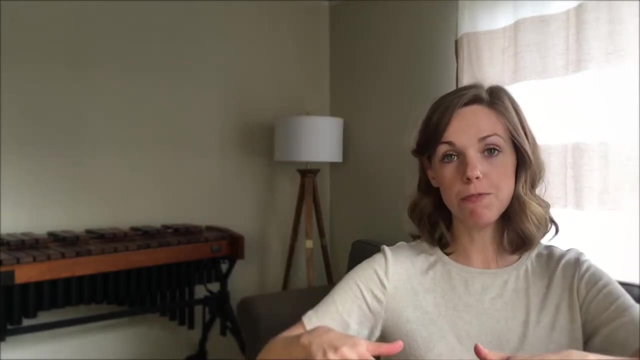 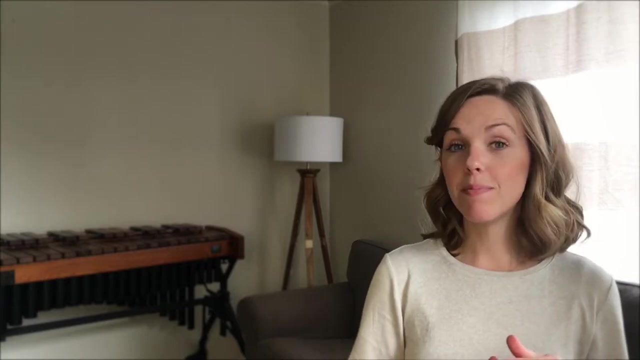 papers. Some students left literally everything blank. Some students went through and circled every single choice. And then there were some students who were able to follow the worksheet flow really well and show me that they could identify musical opposites. But because I asked, 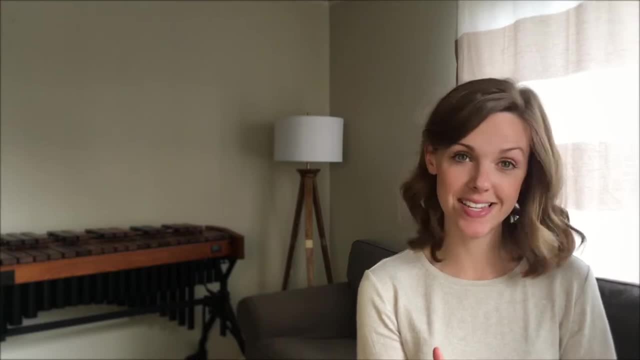 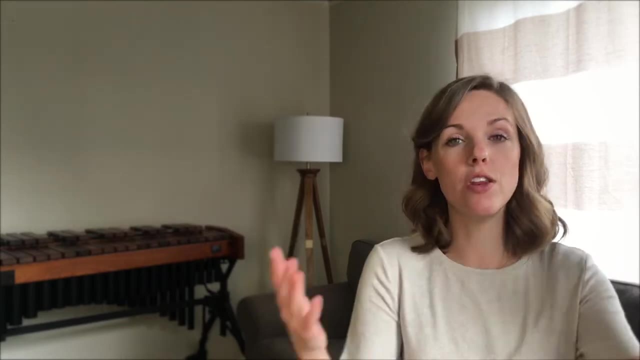 students to show their knowledge in a way that didn't make sense to them. the data I got from that activity was pretty much useless, And it didn't mean that students didn't know their musical opposites. It just meant that I was asking them to show their knowledge in a way. 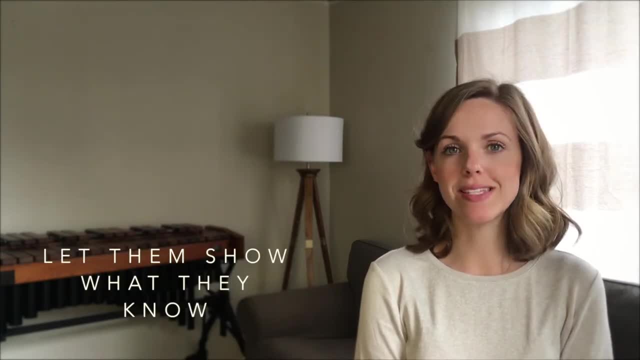 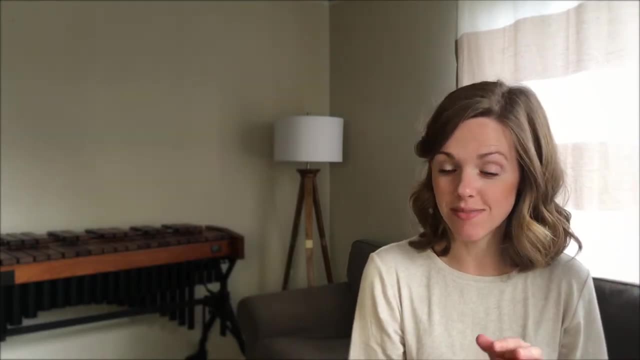 that they couldn't follow. We have to give students assessments that let them shine and show what they know, not assessments that show what they don't know, And there's a big difference. It means thinking through our modes of assessment really carefully. So if you want to do a pitch, 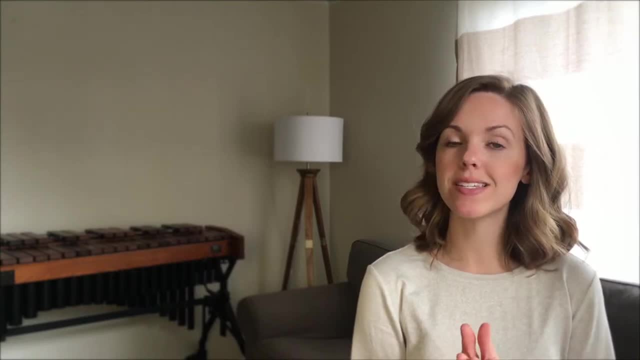 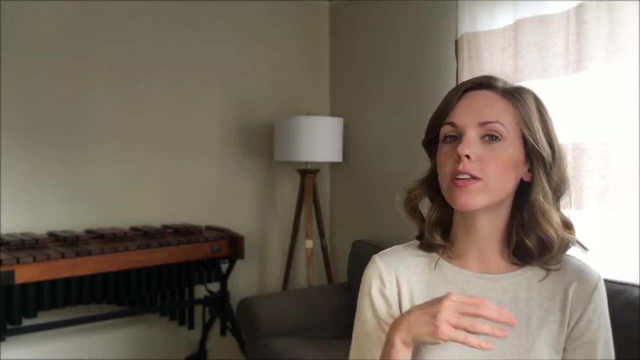 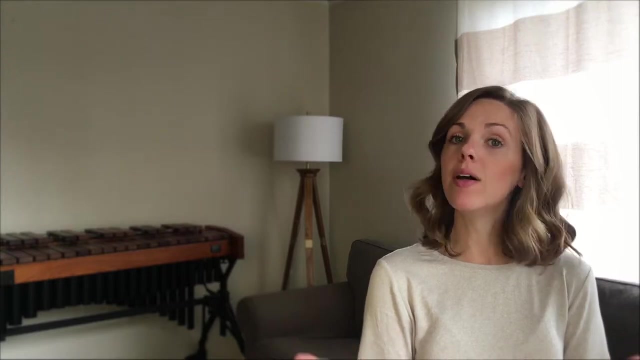 matching assessment for your students and you ask someone to sing in front of their entire class. is that student going to shine when asked to sing, Or are they going to be too shy to really showcase what they can do? The question is, what other modes of assessment can we think about? 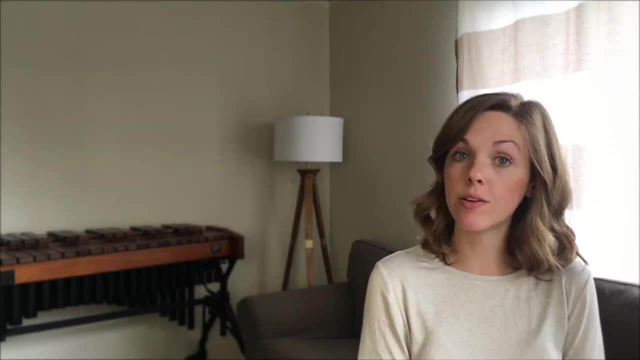 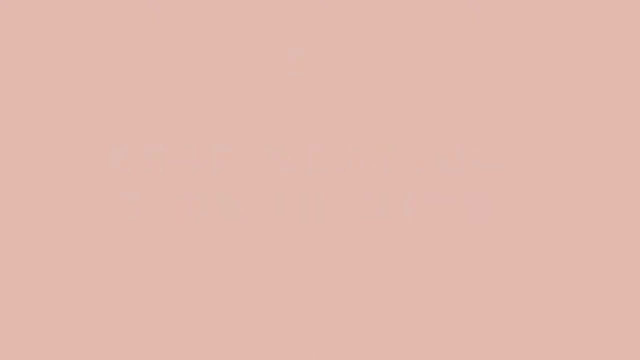 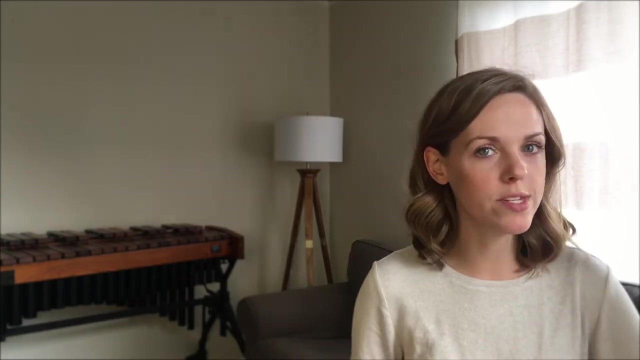 that will give us accurate data. Let's say that you want to give out a really short exit ticket at the end of your music class. That seems like an easy thing to assess because each student is only giving you one response, But you have to think about if you're doing that for a group of third graders. you're 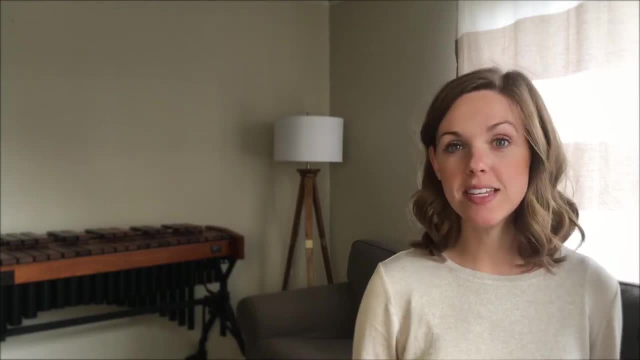 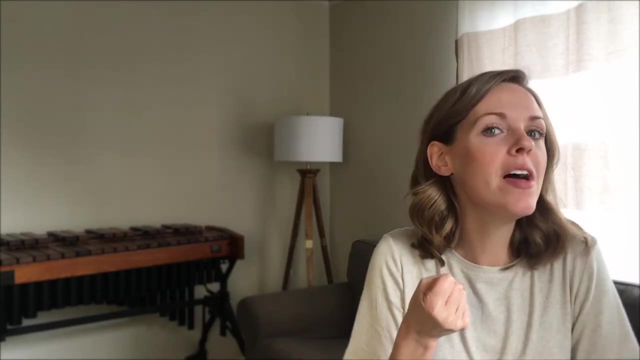 going to have what? maybe four or five third grade classes with what? 20 to 30 kids in each class. By the time you go through even such a simple assessment, you're going to be able to give out a really simple assessment like an exit ticket. You are dealing with so much data. 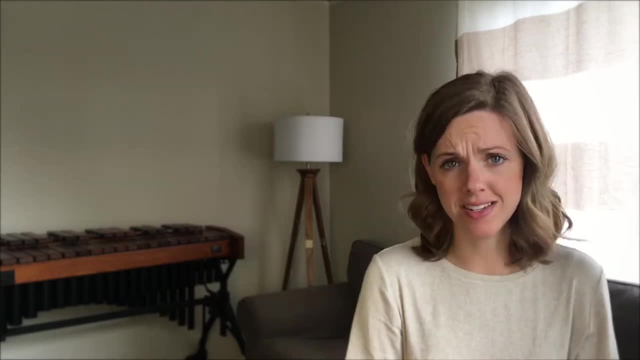 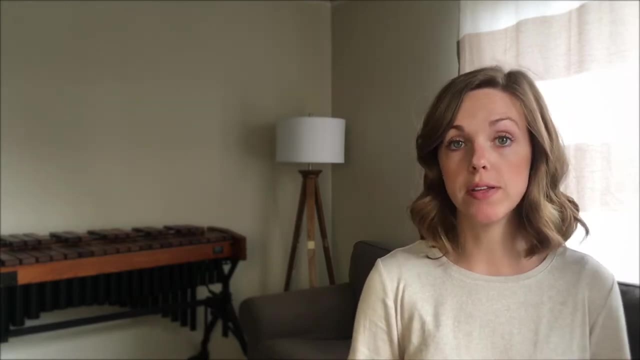 And a short assignment for them to complete means a lot of grading time for you. Or let's say that you're going to test a skill like improvising using quarter notes and eighth notes on Orff-Bart instruments. One thing that a lot of music teachers do here is they will set up a camera. 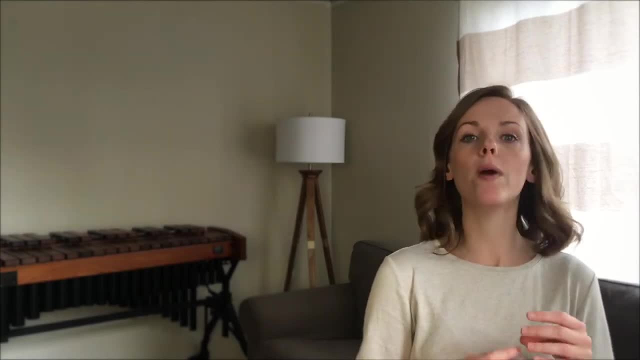 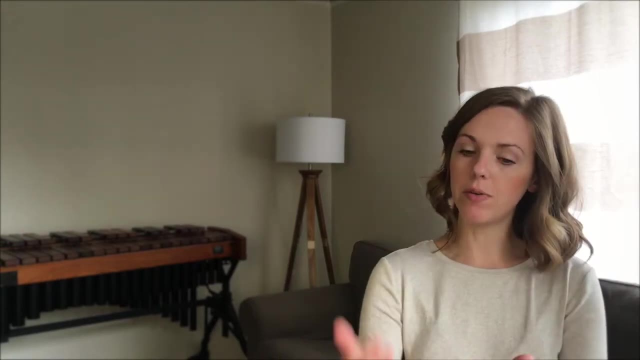 and video their students improvising so that they can still be around to manage the classroom however they need. And then, after the class is gone, at the end of your day, you're going to pull out that video, You're going to watch it and watch each individual student. 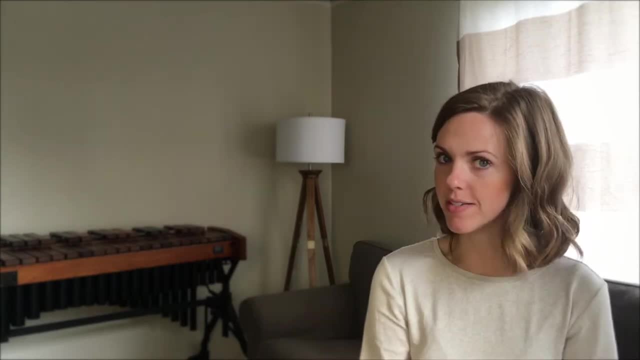 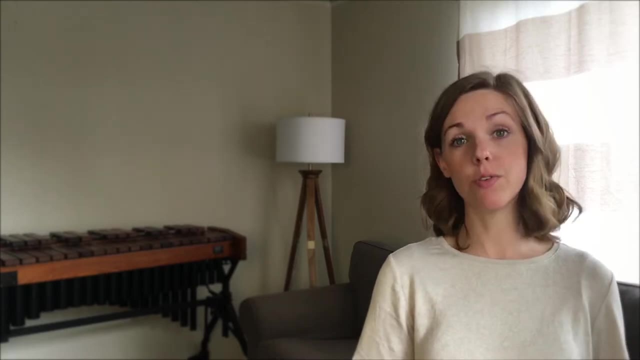 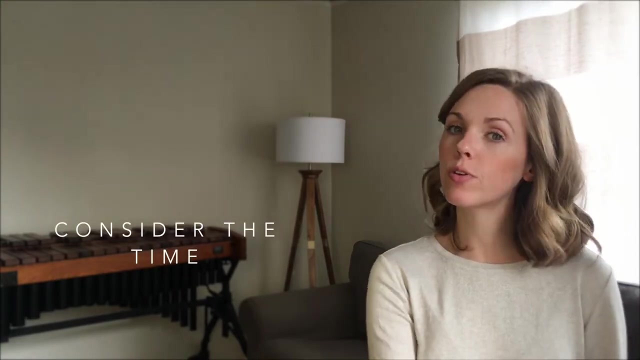 and then record a grade for each individual student. Let's be honest, that takes so much time, And I don't mean that you should avoid doing activities that take time to grade later. I just mean that you need to be prepared for the amount of outside class work that you're going to do when 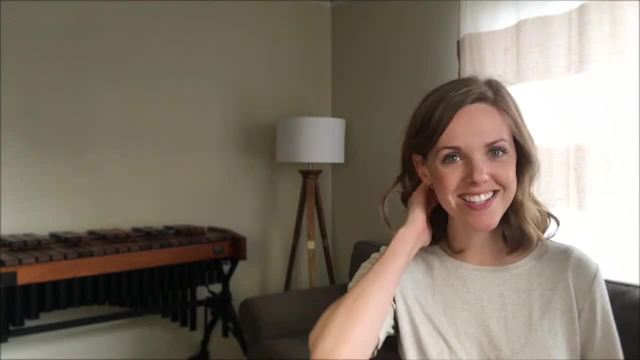 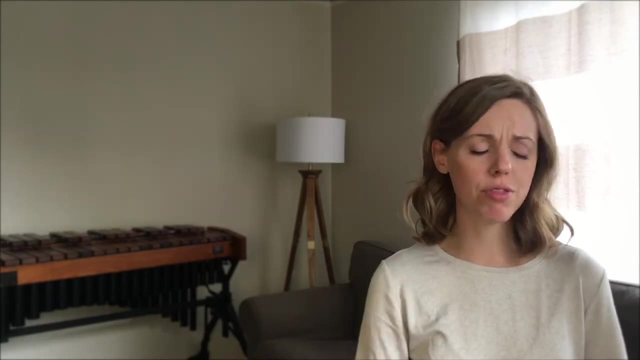 you assign even a really simple activity, I'll be honest and say I've been guilty of biting off more than half of my. so if you want to know how much time you spend doing your desk work- and it may not be enough- it may not be the best opportunity to go through the assessment area. 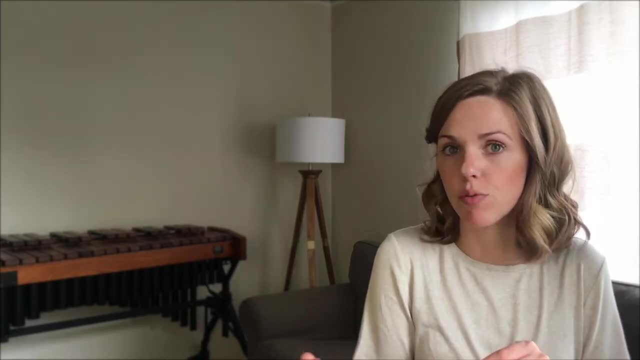 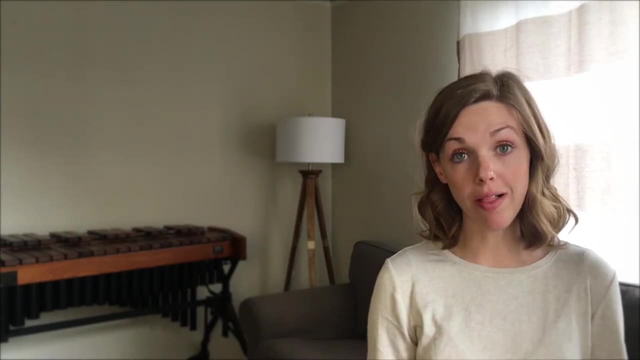 I think that it will be really easy to just go through, But I forget how much time it takes to actually sit through and sift through all that data. I guess all I'm saying here is be aware of the time it takes to do assessments. well, We have to take down information about our students'. 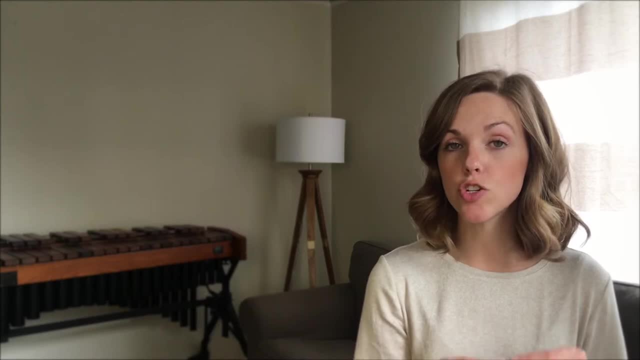 abilities, but it needs to be done in a way that is manageable for us in the short term so that we don't burn out in the long term. Number four is: never, ever, ever, ever do the work of the students themselves. It's important to 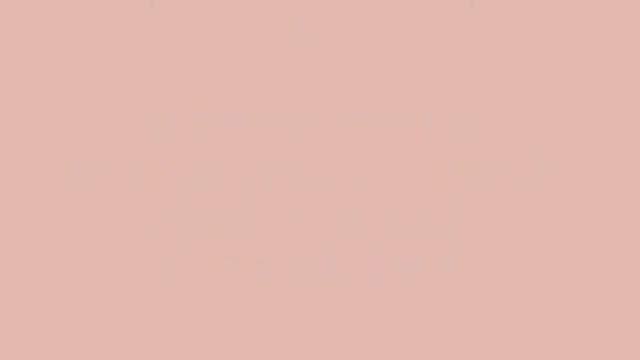 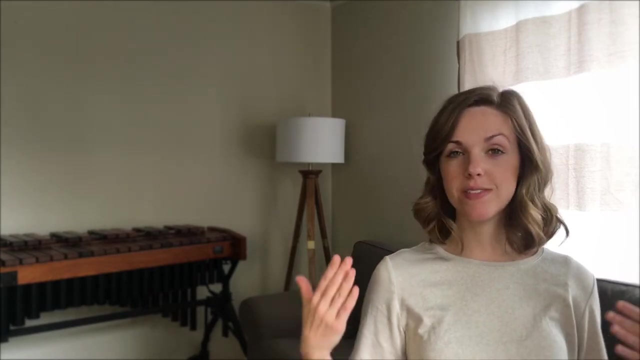 ever, ever embarrass a student in front of their peers. In the early grades, like preschool, kindergarten, first grade, most students are just fine: playing by themselves, singing by themselves, performing by themselves, and it's not a problem. Then we hit around. third grade is what I've. 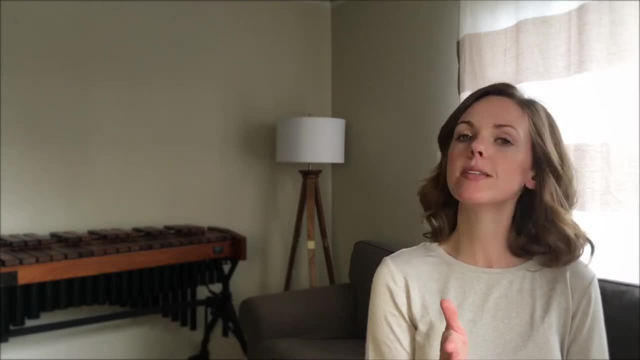 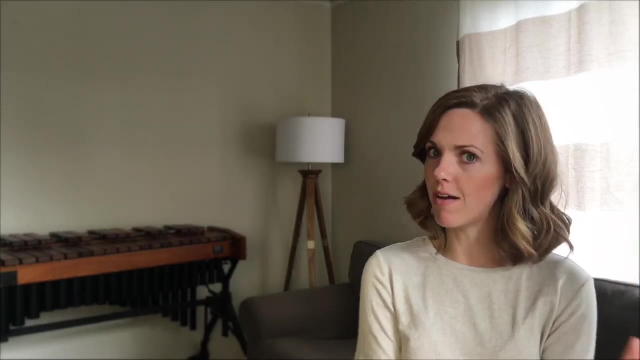 noticed, becomes this kind of tricky area to navigate, Some students decide that music is for them and they're going to love it and it's going to be awesome, And then some kids decide music is not for them, And a lot of times third graders start to develop these attitudes like. 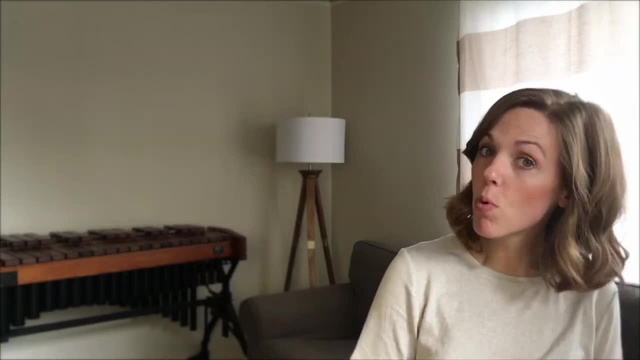 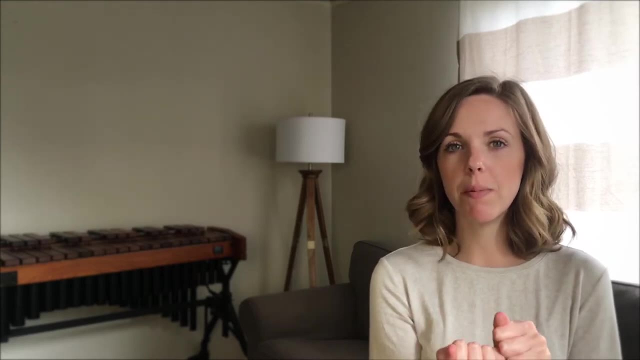 only girls sing. I'm not good at music. I play sports. I don't do music And there's this fear that music is such a public medium. Everyone will be able to tell if I can't do this thing, It's not. 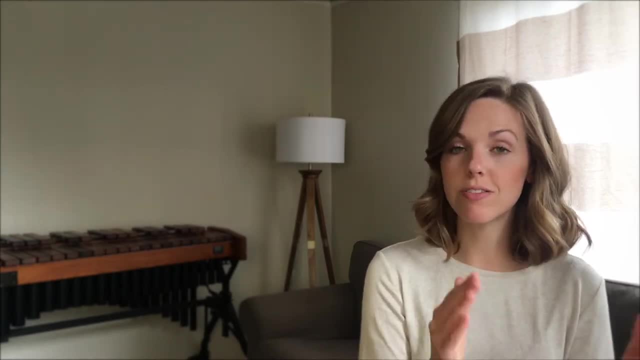 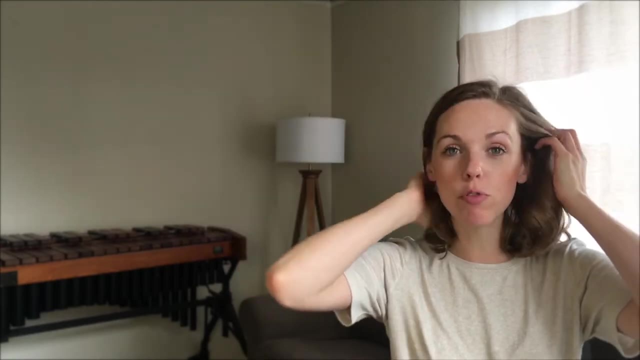 like a paper pencil math test where you record your answers and it's just between you and the teacher. When you do something in music, it is on display for the entire class And that is such a vulnerable point. It's not like a paper pencil math test where you record your answers and it's. 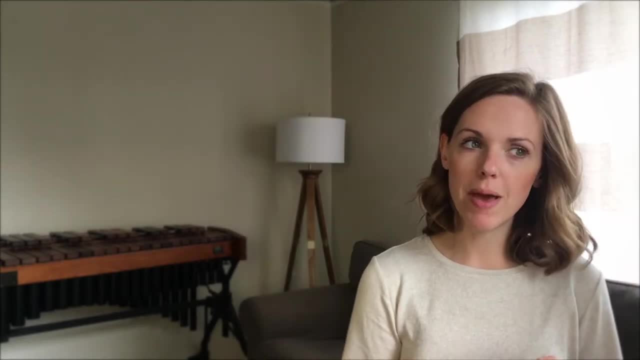 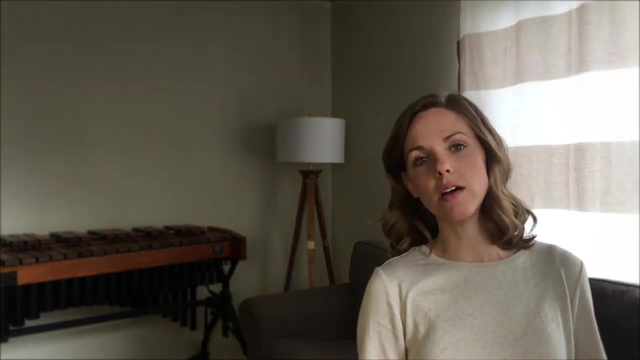 a vulnerable place for us to put our students. We need to be respectful of the amount of courage it takes to do anything performance-based in music. As students become more self-aware, they can also become more self-limiting, and that will change how they perform in our assessments And social 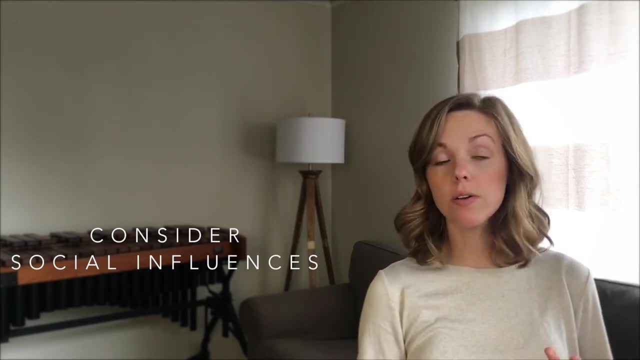 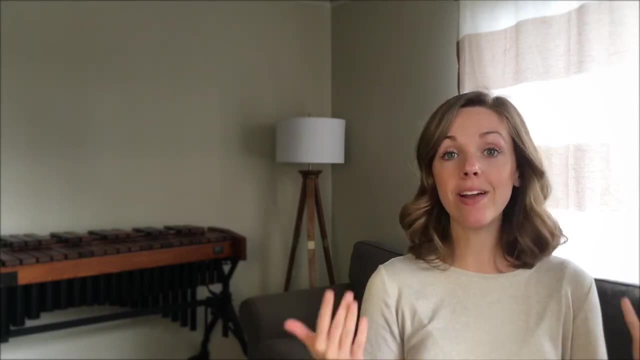 factors play a big part in this. So is music for everyone, or is it only for the talented? If you do sports, can you also do music? Do the kids hear their parents sing at home? Probably not. Let's not forget that music is for everyone, It's not just for the talented, It's for everyone. It's. 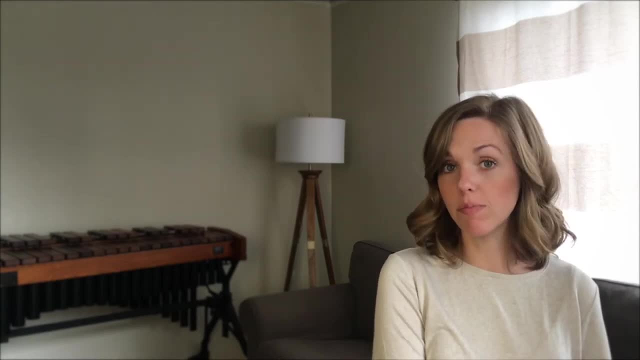 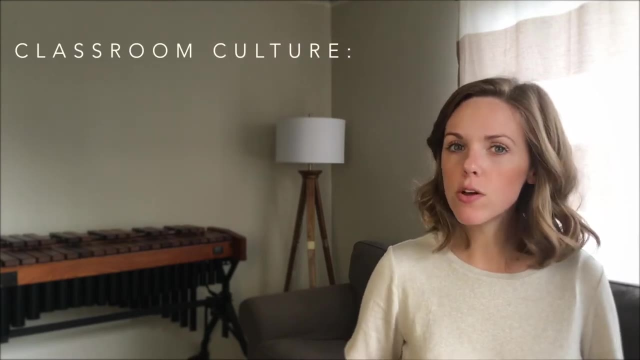 for the kids. We want to get the social influences that students carry into their music class And it absolutely will affect how they perform in assessments. So instead, establish a culture in your classroom where students feel safe and supported. Lay down really strict ground rules. 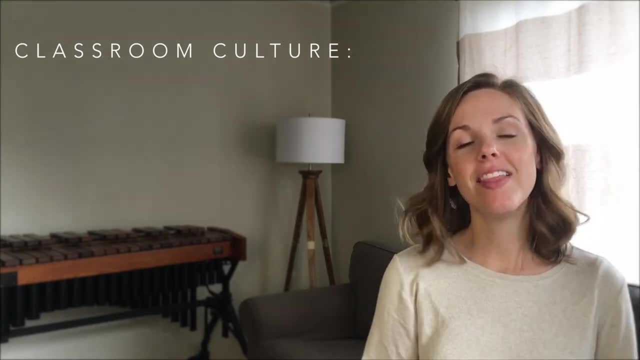 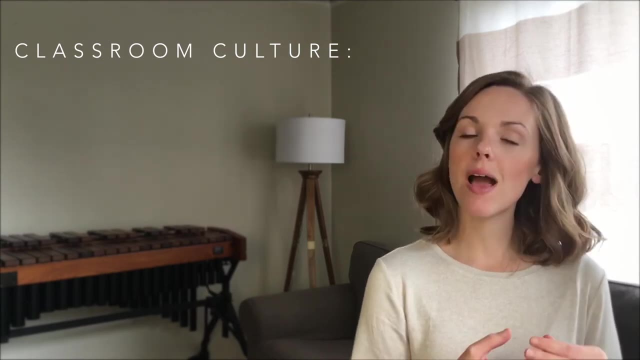 at the beginning, when they're in kindergarten, before they're scared that say: there's never any giggling after someone sings. We only use positive language with our peers, Establish a culture of support and bravery and love, And I think that's a really important thing to do. 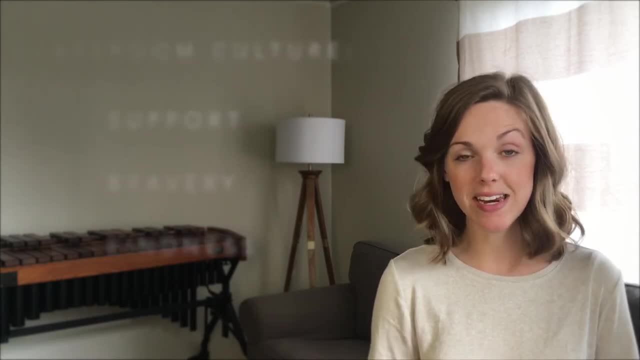 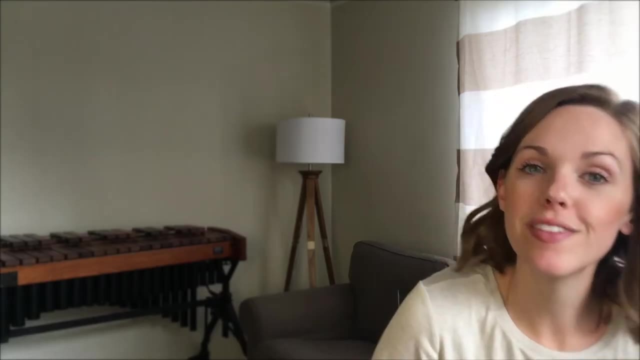 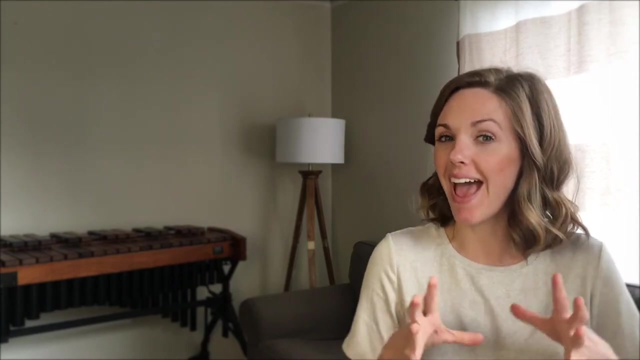 kindness while students are young and still excited about performing. The last thing to keep in mind when talking about assessment is that every assessment is flawed. The sad truth is that there's not an assessment out there that can give you a true, accurate reading of what the student actually understands about the 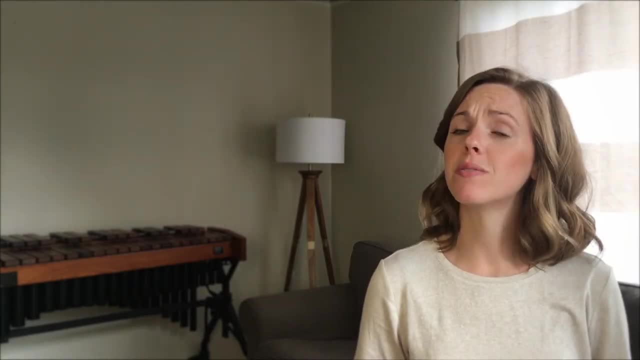 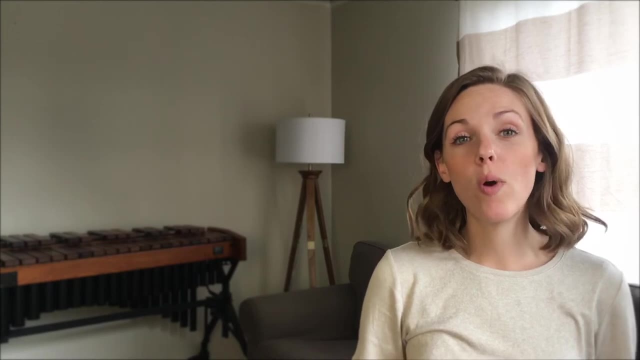 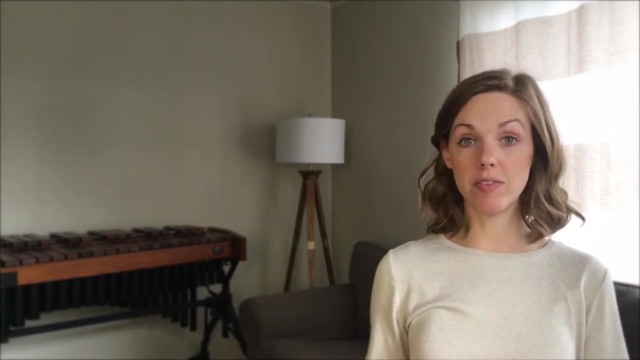 concept. Assessments don't actually tell you if students know the material. Assessments only tell you how a student performs on an assessment. Some students don't perform well under pressure so they might flop when you ask them to echo back a rhythm. Some students might know the comparatives high and low like 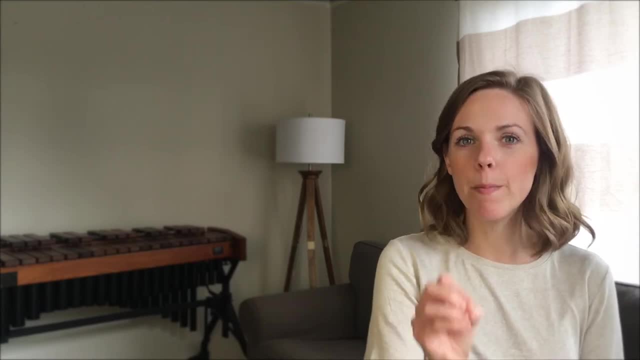 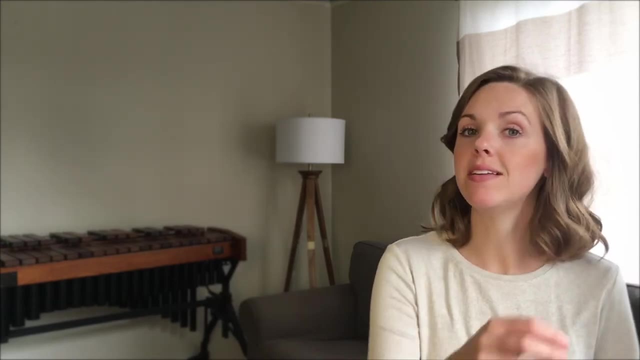 my kindergartners, but not be able to showcase it in the mode that you're asking them. Some students might ace a singing assessment over so and me, but not be able to use so and me in an improvisation. Some students might be able to play a rhythmic element really easily but not be able to recognize it.